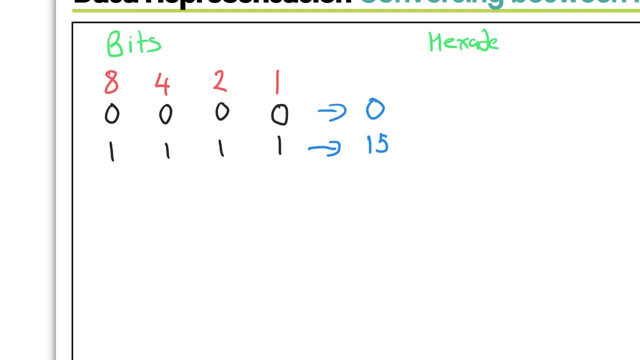 This is with hexadecimal. What's the biggest number we can write down in hexadecimal? Well, that's easy, It's zero. What's the largest number we can make? That's easy, It's F. Well, what is zero in denary? 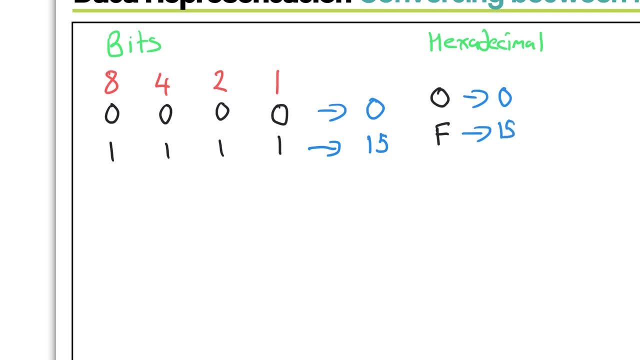 It's zero. What's F in denary? It's 15.. Ah, and there is the relationship: One hexadecimal digit is worth exactly four binary bits, So you can convert directly Every hexadecimal digit. you can convert to eight bits and vice versa. 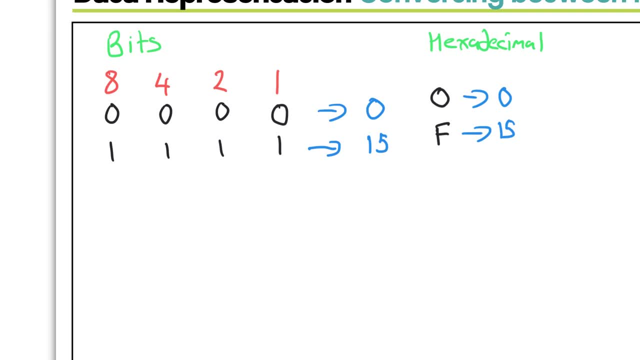 So why don't we try that with a couple of questions? Why don't we just say with a nibble here: 0, 1,, 1, 0.. Okay, Well, the first thing we need to ask is: what number is that? 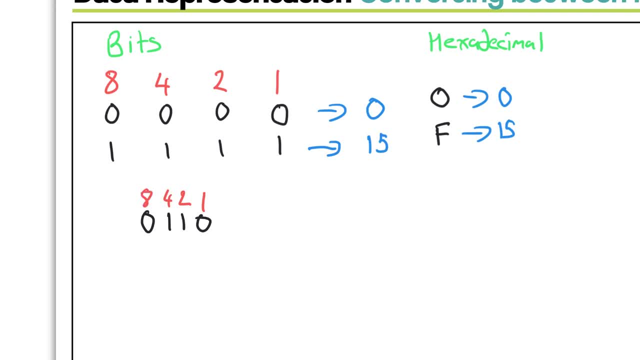 Write out the grid. The number is four plus two, So in hex that would be six. And then we've just converted directly from binary to hex, So binary on this side and hexadecimal on this side. Okay, Let's try a trickier one. 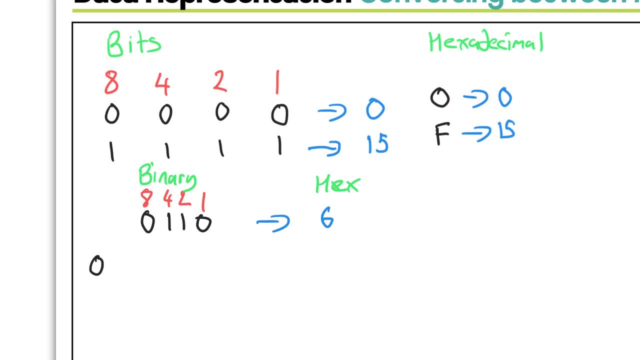 What happens if we've got an entire byte And, if you remember, that's eight bits: 0, 1, 1, 0, 1, 0, 1, 0.. How do we deal with that? 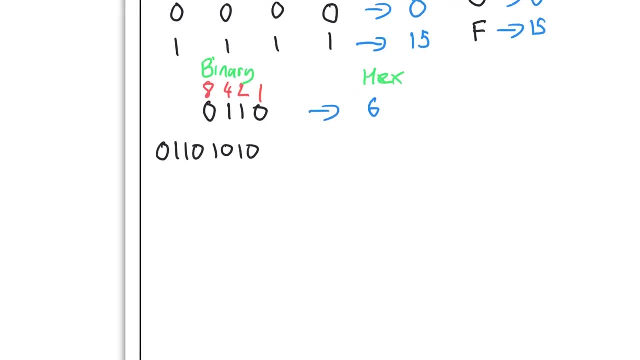 Good question. Well, here's what we do: We split it into two nibbles. So we've got first nibble here, second nibble here. We do the grid again: 1, 2,, 4,, 8.. 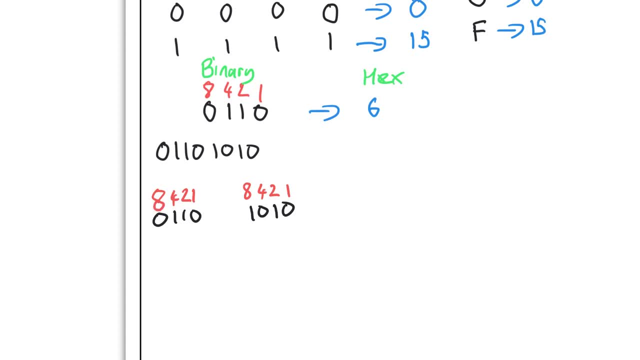 8 plus 4 is 10.. So this is 10 over here. 4 plus 2 is 6.. So it's 6 over here. We know that you can't do 10 in hex, But basically the number will be 6 and 10, which will be A. 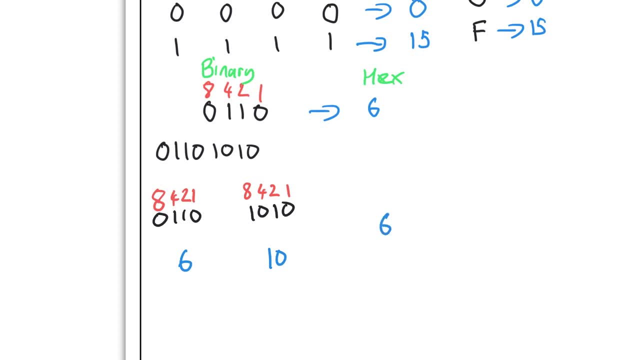 And you can write down 1, 16.. So what is 0, 1, 1, 0, 1, 0, 1, 0 in hex? Well, you can write down 1, 0, 1, 0, 1, 0 in hex. 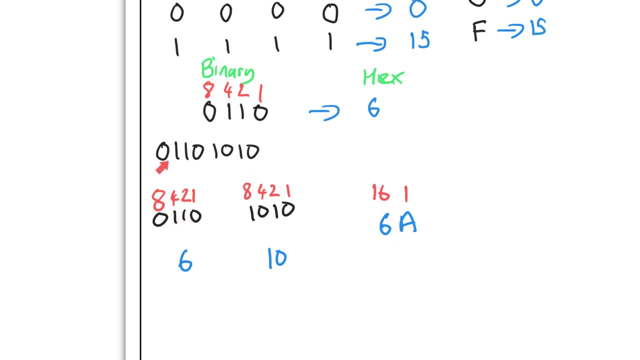 It's 6A, because the first set of four bits 6,, second 10.. And then, if we wanted to convert it back, we could do it the other way around as well.